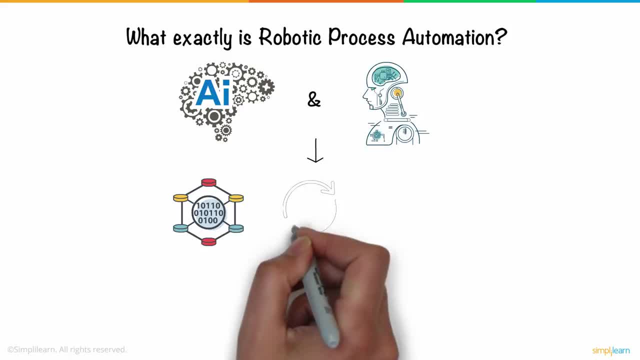 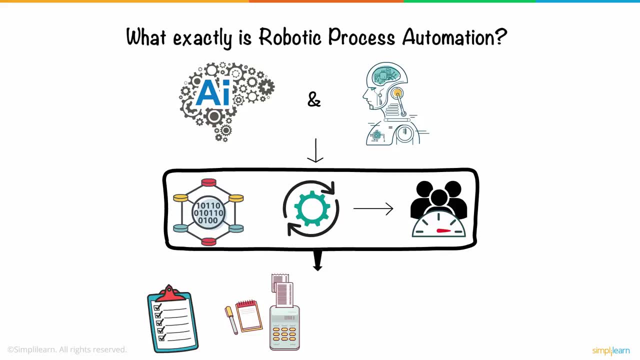 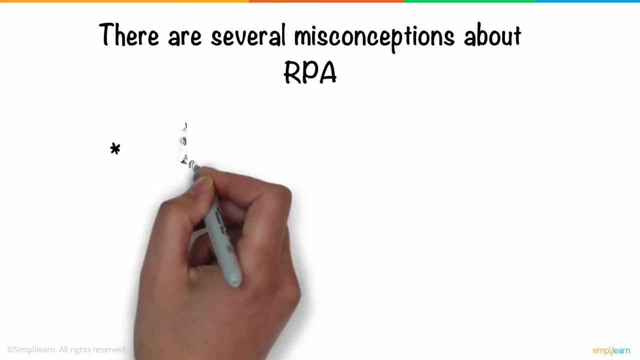 and machine learning capabilities to handle high-volume, repetitive tasks that previously required humans to perform. Some of these tasks include addressing queries, making calculations, maintenance of records and more. So what exactly is Robotic Process Automation? There are several misconceptions about RPA. RPA is not a humanoid robot. It does not have a physical 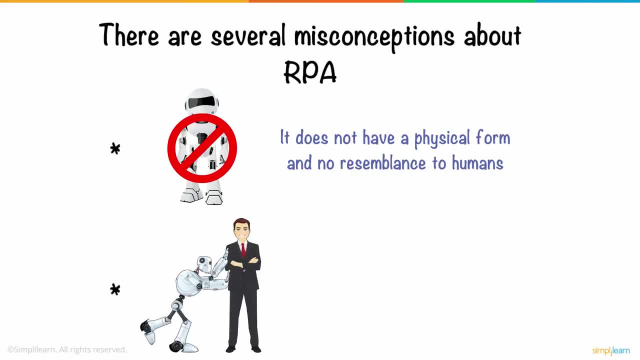 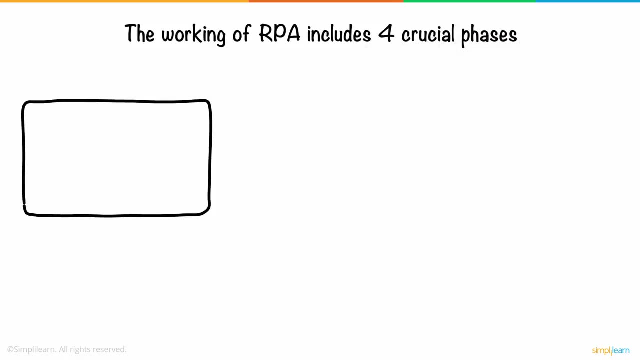 form and no resemblance to humans. RPA cannot replace humans or replicate human cognitive functions. It does not have a brain of its own And cannot perform logical or critical thinking as humans do. The working of RPA includes four crucial phases: 1. The planning phase typically involves gathering the processes. 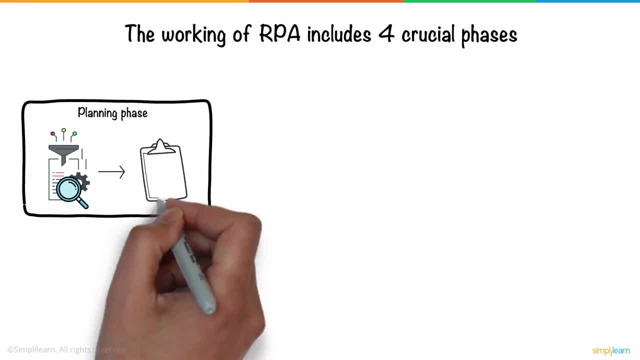 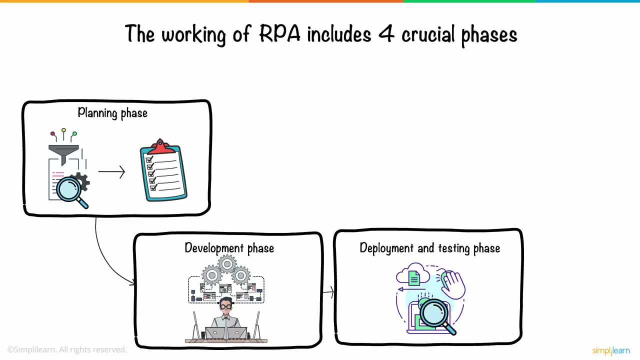 to be automated, identifying the test objects and finalizing the implementation approach. 2. The development phase includes the creation of automation workflows as per the agreed plan. 3. Deployment and testing is a vital phase, since it uncovers any unexpected outages and ensures a 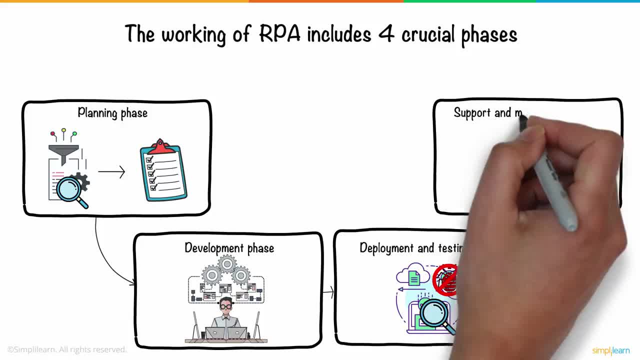 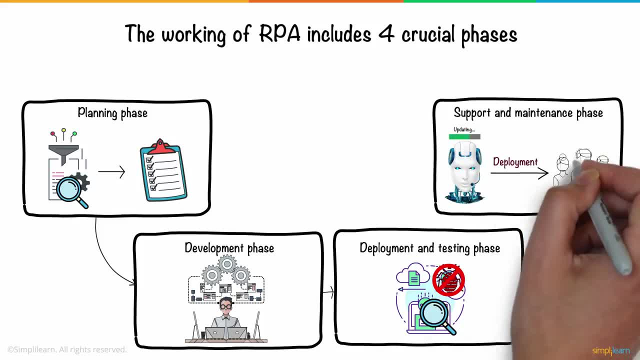 bug-free product 4.. Lastly, there's the support and maintenance phase, which ensures that the product is continuously updated with smooth deployment across the userbase. To meet the objectives of RPA tools are used. These RPA tools are software applications. 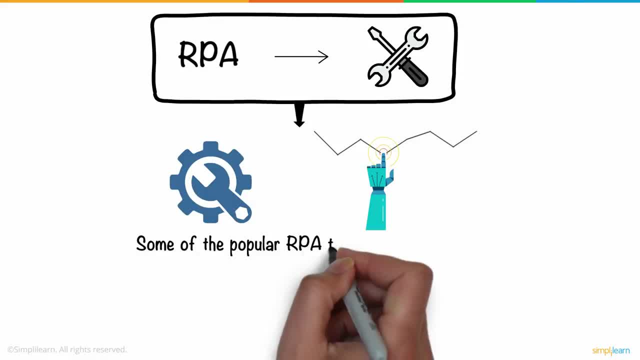 that can configure tasks and automate them. Some of the popular RPA tools in the market are UiPath, Automation Anywhere, BluePrism, WorkFusion, Pega and Redwood, among others. They are a good reward. A vizing of RPA is thus articulated. 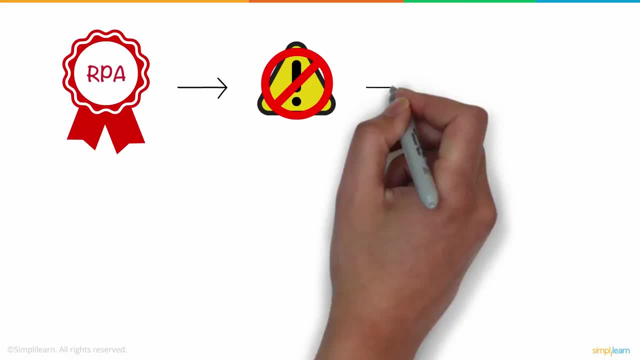 O2 is stackable and inexpensive according to new safety standards by numbers and international stores, but of course you just needál toma McDonald. When it comes to quality, RPA ensures consistent, error free output leading to reduced operational risks. This in turn improves customer satisfaction in the market. In the area of delivery, RPA is a commanding tool for the RPA systems with 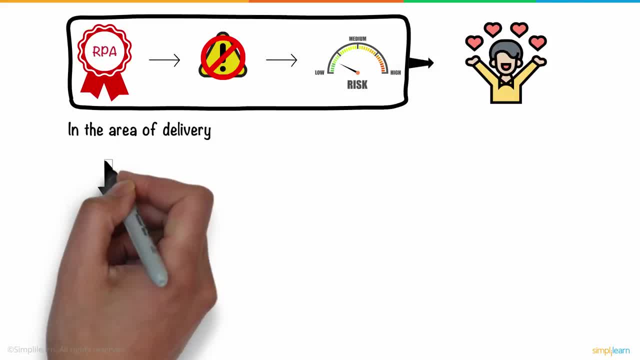 clients because RPA ammo files are strong for student blackboards. This US primary customer handling technology In the area of delivery, RPA, can help decrease the average handling time and this enhances the customer experience and ensures 24-7 business continuity. With respect to cost. according to NASSCOM, domestic businesses can reduce the cost by up to 65% through RPA. It offers a higher ROI by driving positive returns within quarters as opposed to years. Other advantages of RPA include reduced training costs, minimal utilization of IT. 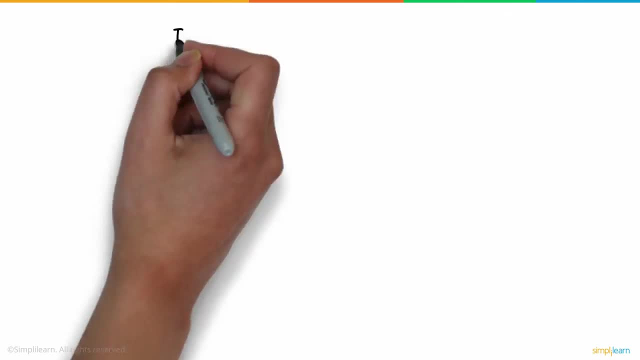 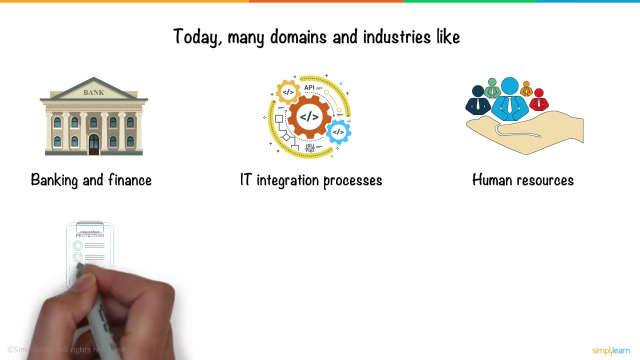 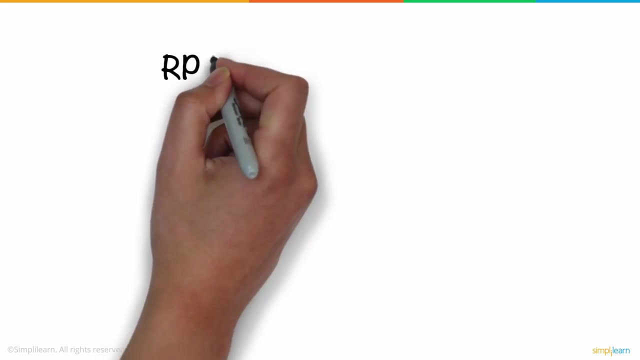 resources and easier software migration. Today, many domains and industries like banking and finance, IT integration processes, human resources, insurance agencies, marketing and sales and customer relationship management readily deploy RPA. RPA service adoption has been showing tremendous growth since 2016 and will continue to increase beyond 2020.. According to McKinsey's research, knowledge in work automation could have an economic impact on business performance and it could be a key factor in the growth of RPA Of $5-7 trillion by the year 2025, it will impact more than 230 million knowledge workers.